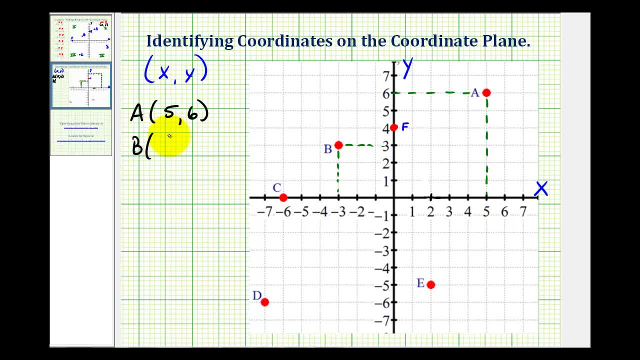 So point B has coordinates negative three, positive three. Now point C is a little bit different. Notice how it lies on the x-axis. So we can see the x-coordinate is going to be negative six. And if we draw a segment straight to the y-axis, 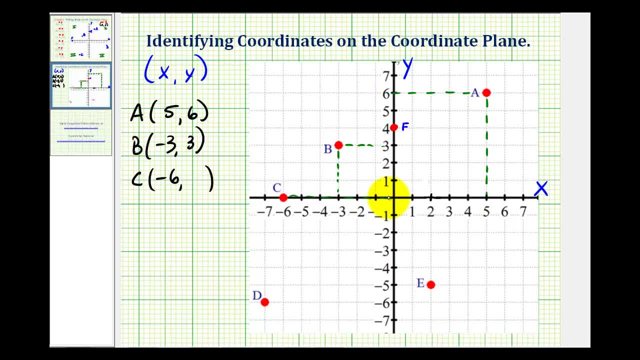 notice how it would intersect the y-axis right at zero, and that's because this point does not move up or down from the x-axis, So the y-coordinate is zero. Now let's take a look at point D down here in the third quadrant. 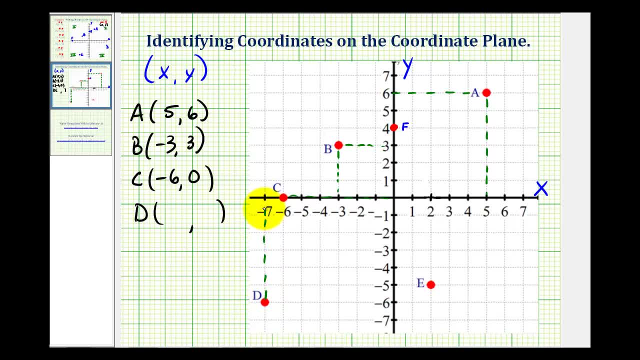 If we draw a segment straight to the x-axis, notice how it intersects the x-axis at negative seven. If we draw a segment straight to the y-axis, it intersects the y-axis at negative six. So the coordinates for point D would be negative seven comma. negative six. 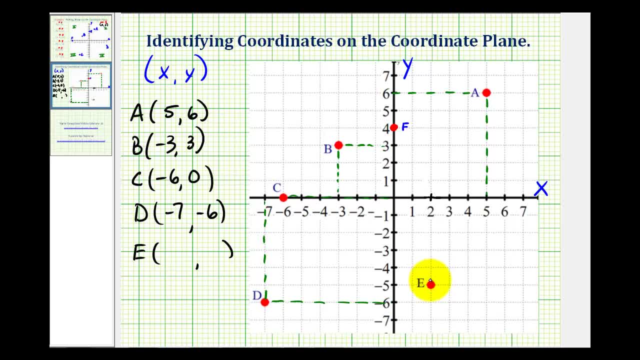 And then for point E, if we go straight to the x-axis, it intersects the x-axis at positive two, And if we draw a segment straight to the y-axis, it intersects at negative five. So the x-coordinate is positive two and the y-coordinate is negative five. 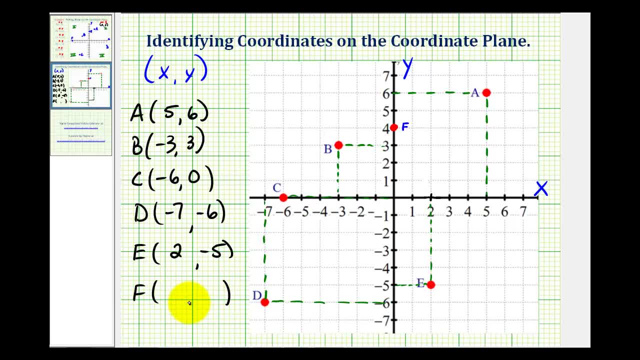 And for the last point, we have point F, which lies on the y-axis. So if we drew a segment straight to the x-axis, notice how it intersects the x-axis right at zero. So the x-coordinate is zero And then we can see the y-coordinate would be positive. four: 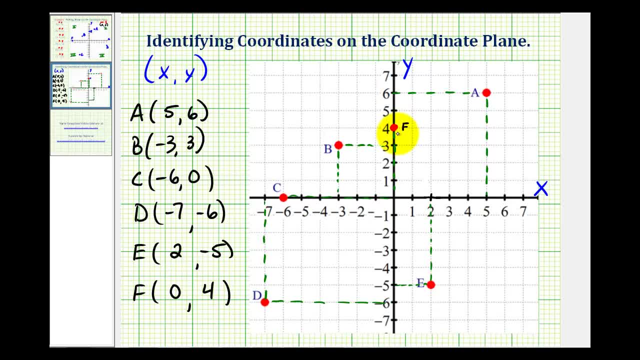 So notice how, when the point lies on the y-axis, the x-coordinate is always going to be zero, And when a point lies on the x-axis, like point C, the y-coordinate will always be zero. And then one more thing that I do want to mention. 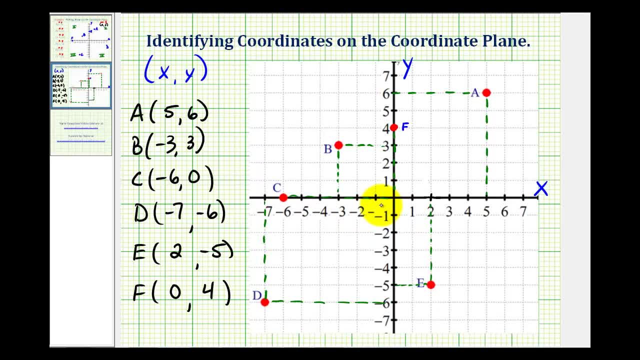 there are four quadrants in the coordinate plane formed by the intersection of the two axes. This is the first quadrant, this is the second quadrant, third quadrant and fourth quadrant. So in the first quadrant both the x and the y-coordinates. 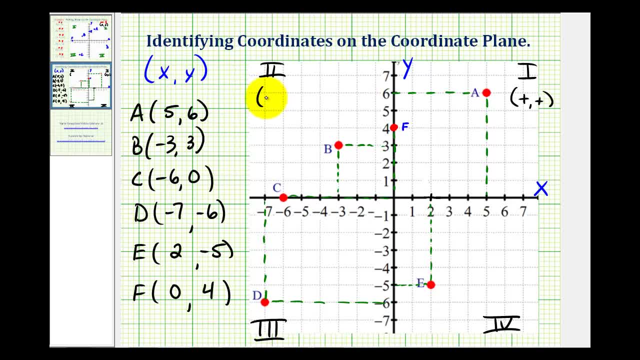 are positive. In the second quadrant the x-coordinate is negative, the y-coordinate is positive. Third quadrant: both coordinates are negative. And the fourth quadrant the x-coordinate is positive and the y-coordinate is negative. So point A is in quadrant one, point B is in quadrant two.